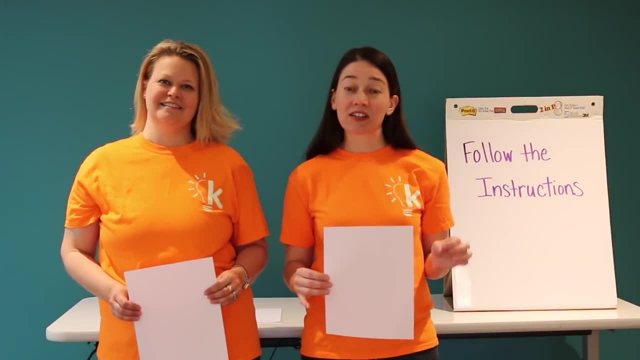 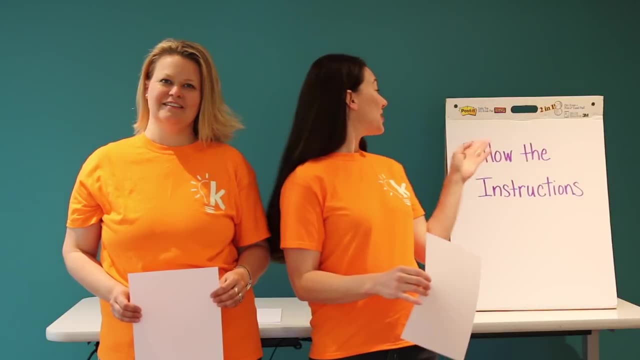 them solve the specific challenge of showing students that there is more than one right answer for the same problem. So today we're going to introduce you to an activity ironically named. Follow the Instructions. All you need is simple: 8.5 by 11 paper and less than three. 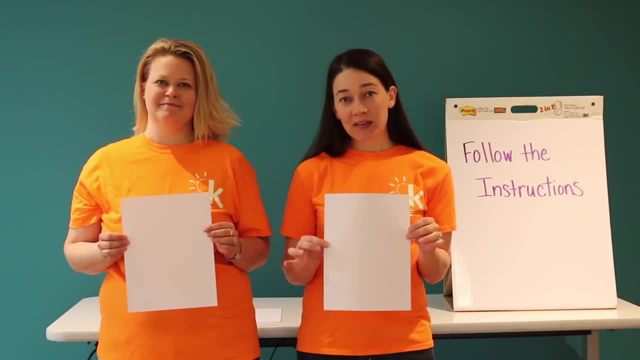 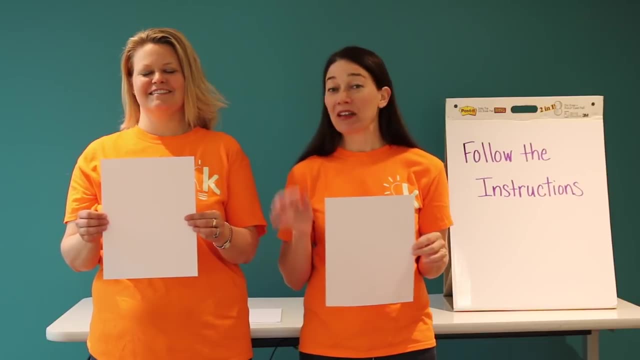 minutes to do the activity. It goes like this: Pass a piece of paper out to every student in your class. Ask them to stand up, hold the paper in front of them like this and close their eyes. Make sure they have their eyes closed. That's key to this activity being 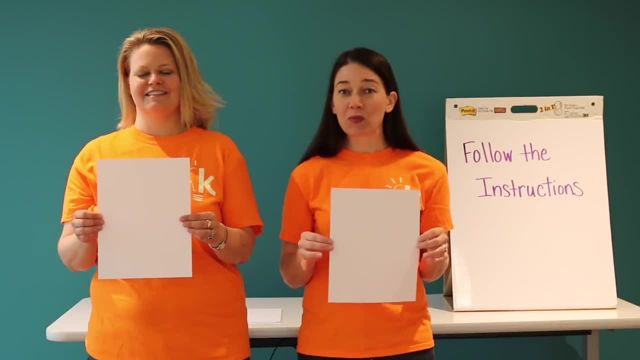 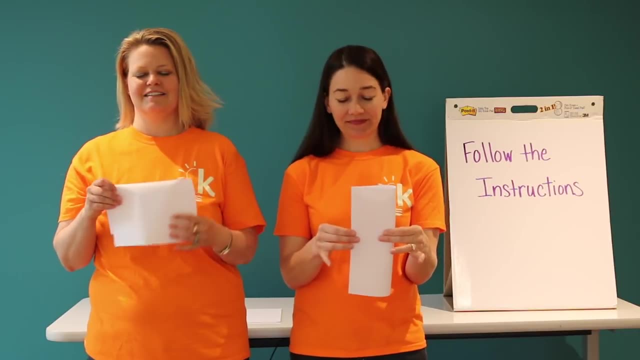 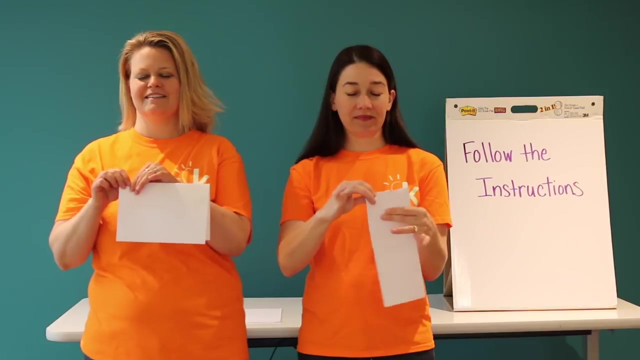 a success. Then you're going to give them a few simple verbal prompts and they follow the instructions. It begins with folding the paper. Fold the paper in half. Now ask your students to tear off the upper right-hand corner of their paper. Ask them to fold in. 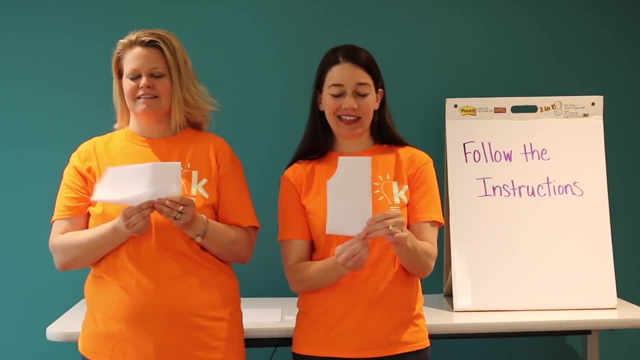 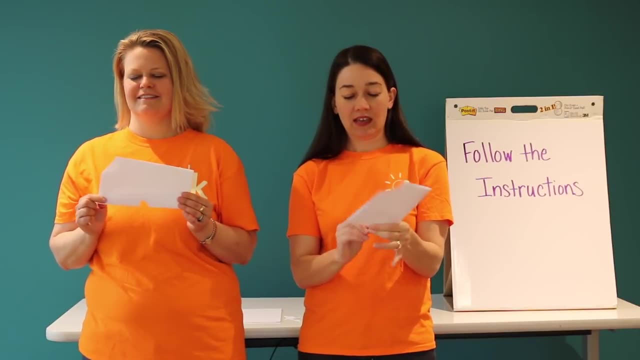 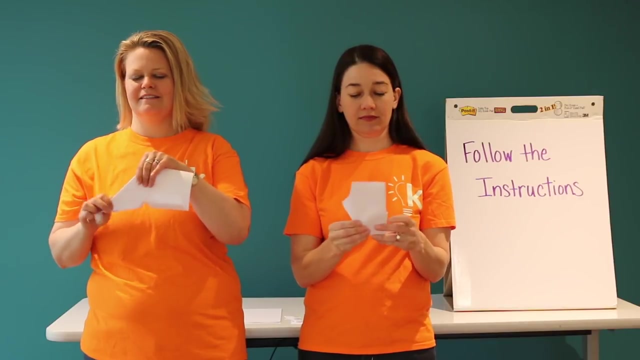 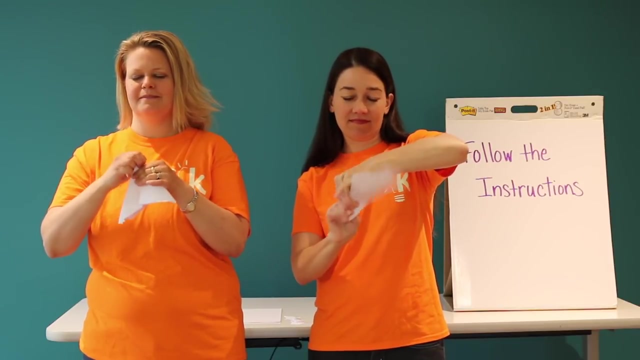 the bottom edge, Make sure their eyes are still closed And then tear off a section along that bottom edge. Now fold the paper into a triangle And then instruct the kids to tear off one of the points of the triangle. Finally, ask them to turn the paper over and tear off a portion along 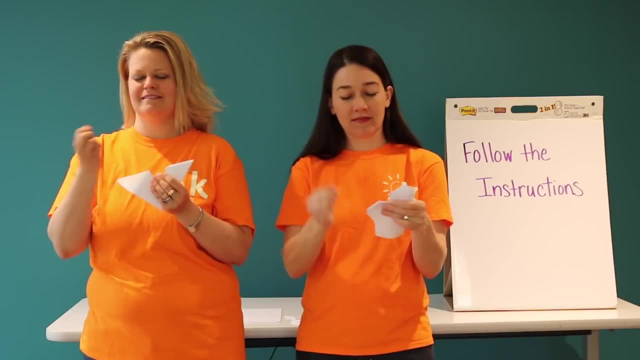 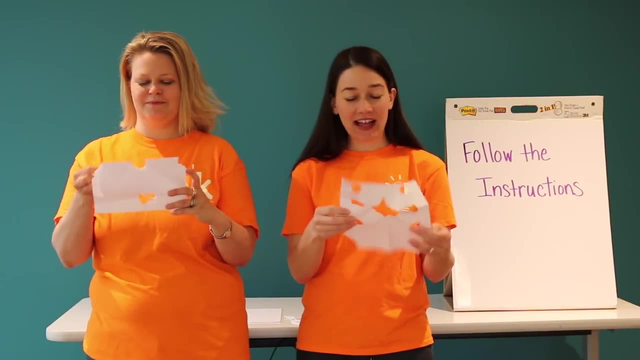 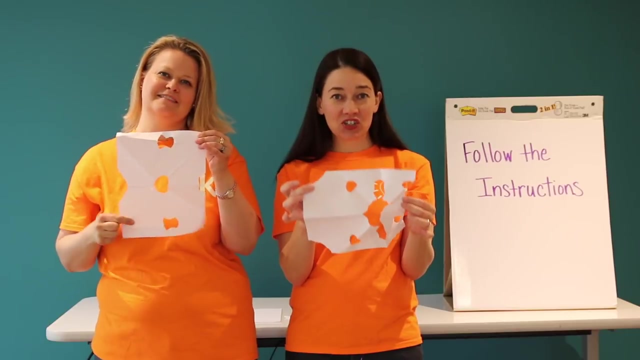 the top edge. Ask them to open up their paper And open up their eyes As they look around the classroom. it will be obvious to see how different all of the papers look By following the exact same instructions. there were numerous different solutions. This activity is an easy and efficient way to show kids that there 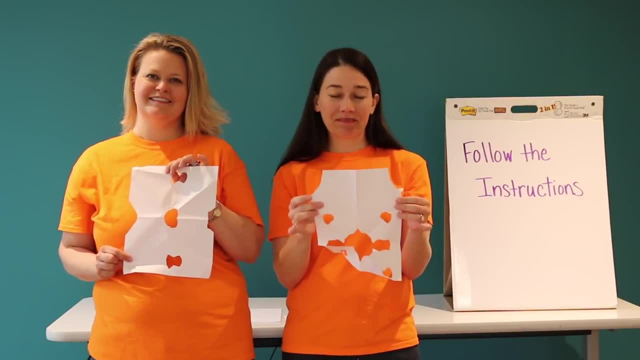 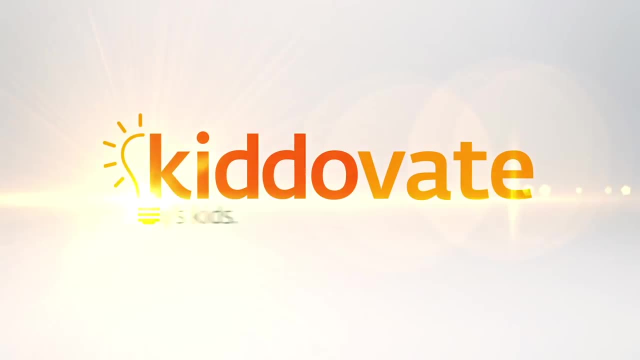 are many more than one answer to a simple problem. We hope you enjoyed the activity. Let us know how it goes in your class. Thanks. Subtitles by the Amaraorg community.